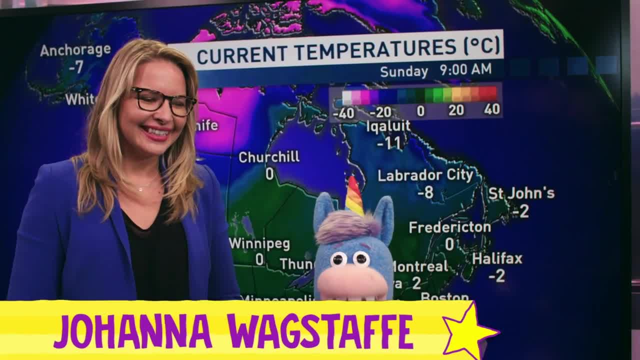 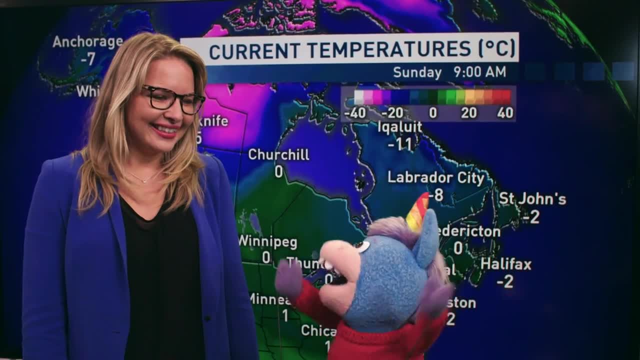 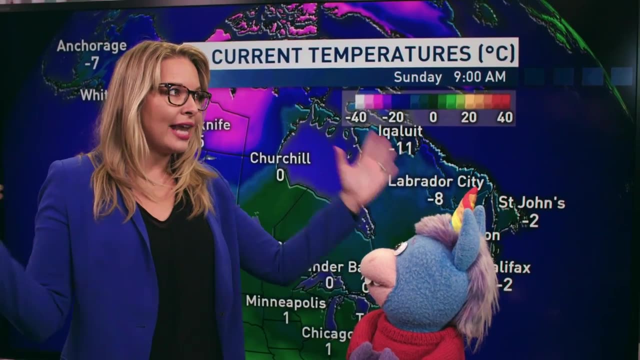 Oh, oh, Joanna, Everybody. this is Johanna Wagstaff and she's the meteorologist of CBC Vancouver. Meteorologist, who would have thought of that? Thank you, I have no idea what a meteorologist is. That's fair. That's fair, Gary. So a meteorologist studies what's going on in the atmosphere around us. 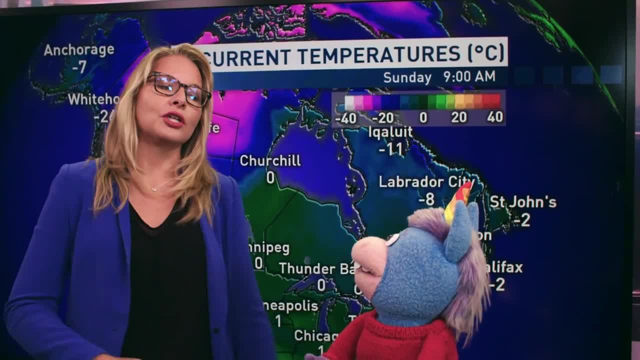 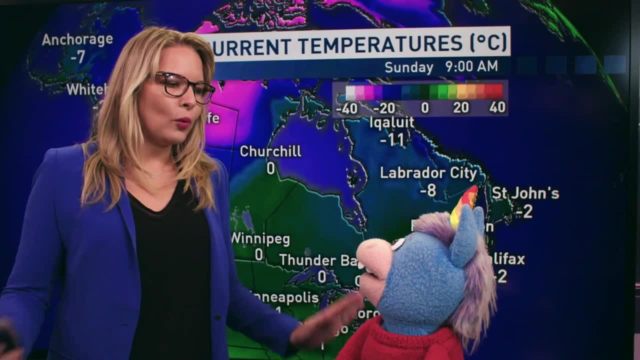 to make a prediction about what the weather will be in the future. You can tell what weather's going to come. I sense rain, And then rain happens. It's even better. I do it with science. So what is it behind us here? 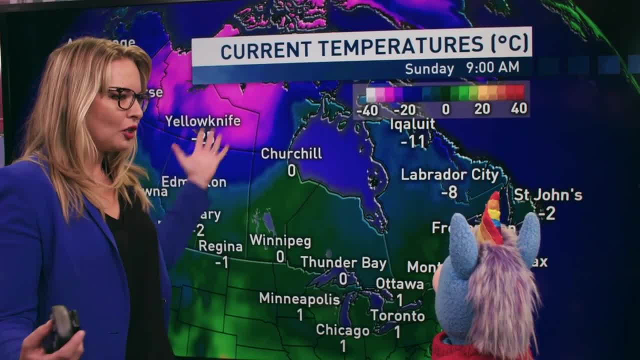 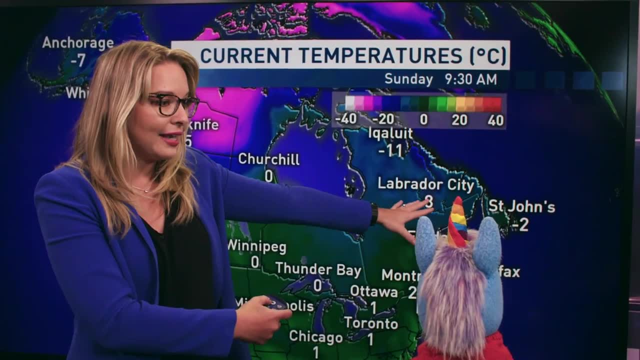 So this is the temperature map. So this really tells me what's going on across the country, And things generally move west to east. So if I know what's happening in the west, I know it's going to eventually end up on the east side of the country. 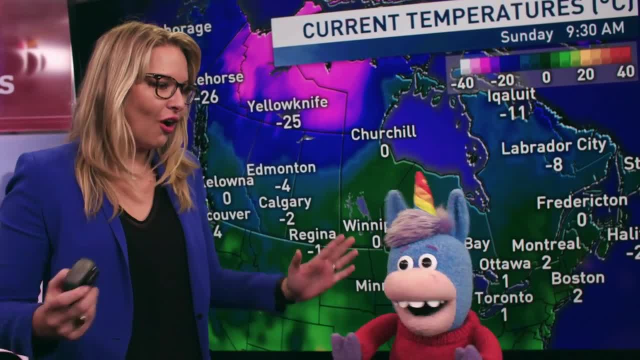 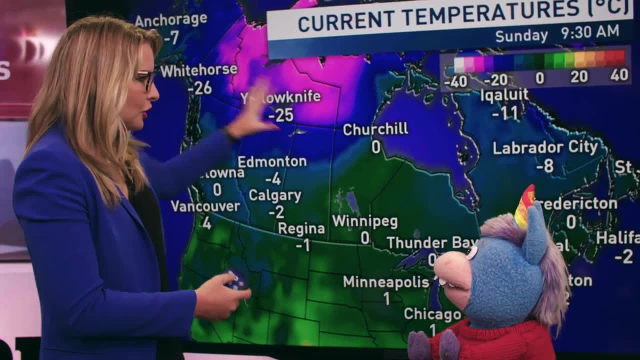 Wow, Can you show me how to do the weather now? Yes, All you have to do is point to what's happening on our temperature map right now and make sure you tell everyone across the country what it's going to be like today. For the best weather reporting, you have the best team here on CBC. 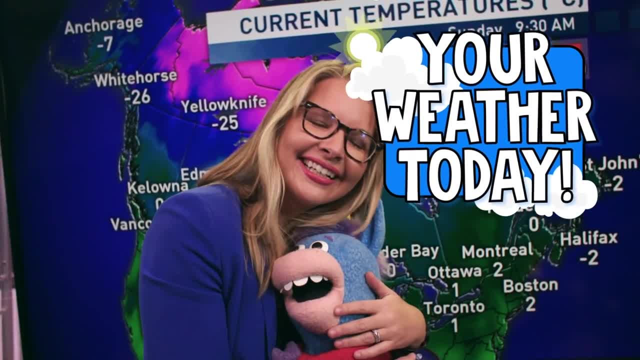 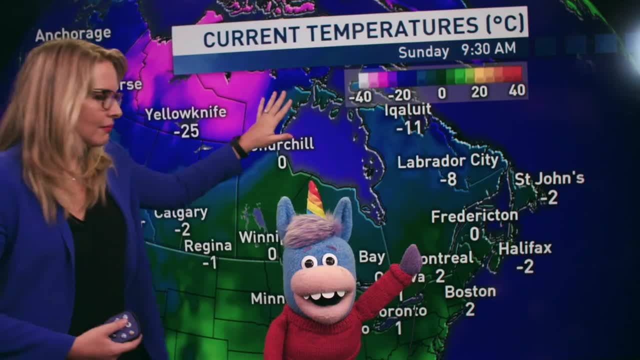 It's Gary and Jo and we're doing the weather, And your weather today is cotton candy, a big blob of cotton candy all over Yellowknife. There's a rainbow over top of Iqaluit right now. Jo, this is the most amazing thing I've ever done. 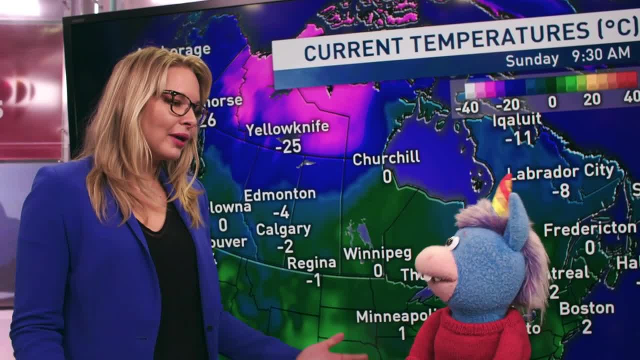 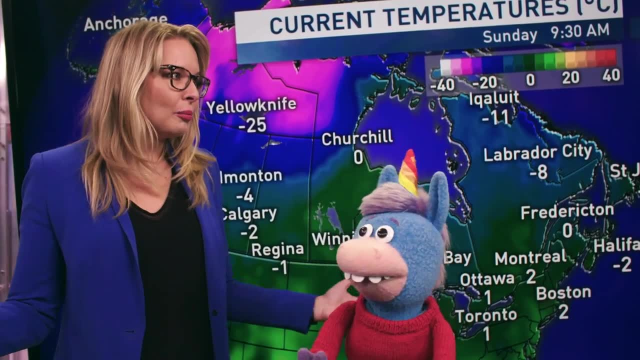 And thank you so much for telling me how to be a meteorologist- Well, it was so nice to have you- and thanks for giving me some tricks to make people happier with their forecasts. Weather is kind of important, isn't it? I think it affects every single person every single day around the world. That's why I love it so much.